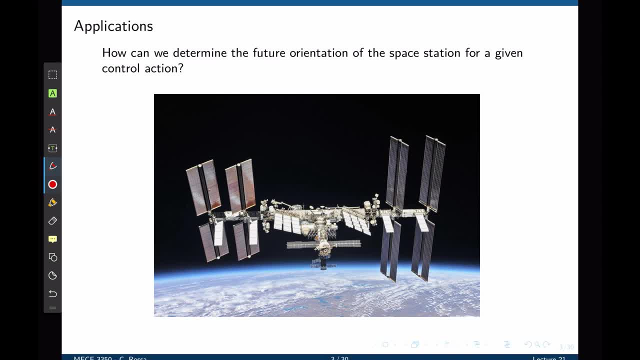 equations. We are not going to formally address modeling in this lecture. We are going to use the principles developed in lecture 2 to come up with time-invariant state equation models of these physical systems and represent them using matrices. This is one example of state-space model. How can we determine the future orientation? 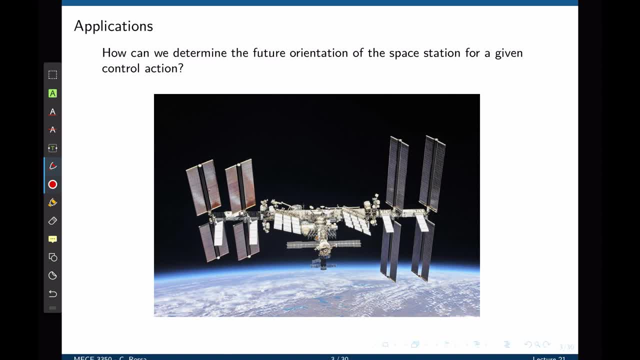 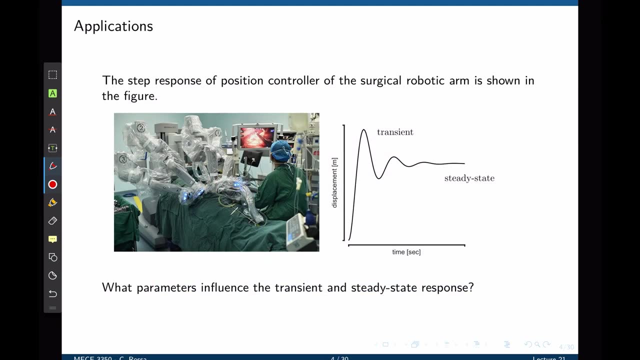 of the space station. We need to know the current state of the system and the inputs to the system. In other words, how does the input affect the future state of the system, given the current state of the system? Here is another example. Consider the step response of the position controller of this. 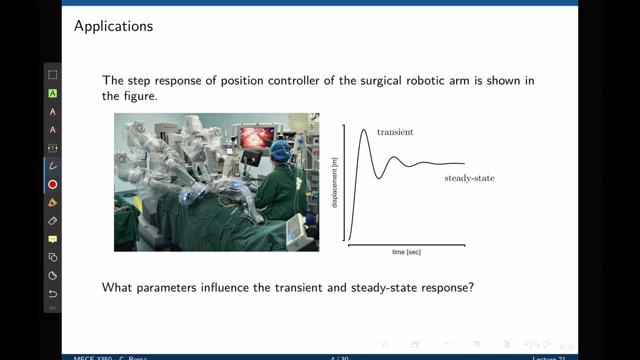 robotic arm. What parameters influence the transient response and steady-state response of the system? How can we highlight them more explicitly? How can we find the relation between the current states, the input and the state In order to represent the state-space variables? we need to define what the state of a system. 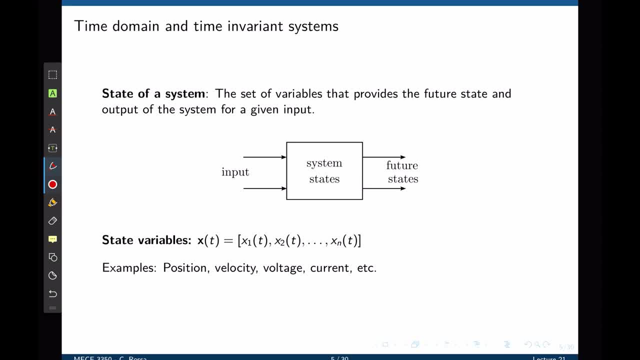 is A state of the system, is defined as the set of variables that provides the future state and the output of the system for a given input. For example, consider a mass spring damper system. The input could be a force applied to that system In order to predict the output. 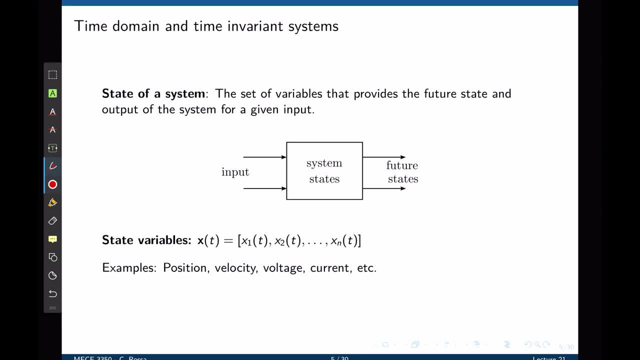 say the position. one must know the current position of the system and also the current speed of the system. The position and the speed are dependent on each other, While the current states of the system, The input is the force and the output are the future states that 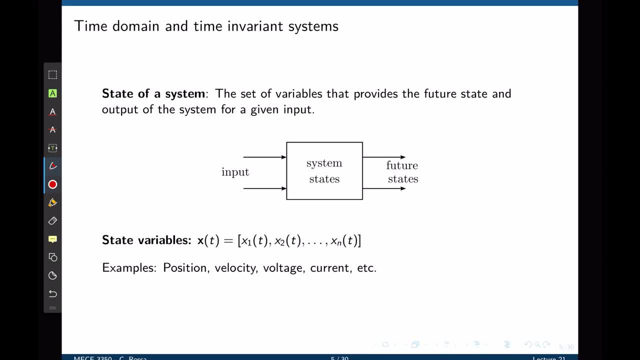 is, in this case, position and speed. We can now define a set of variables that will be represented as a vector, and these variables are the states of the system, For example, position, velocity, voltage and current. Typically, the state variables are the minimum set of variables that are required. 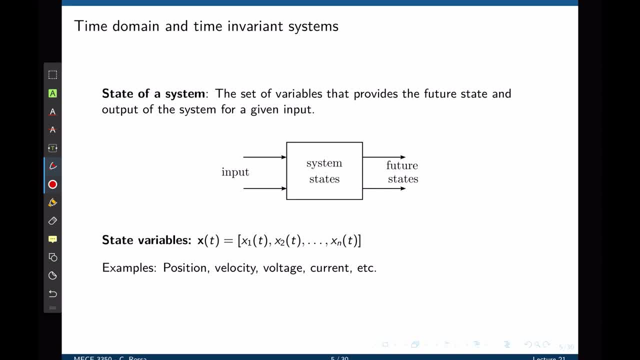 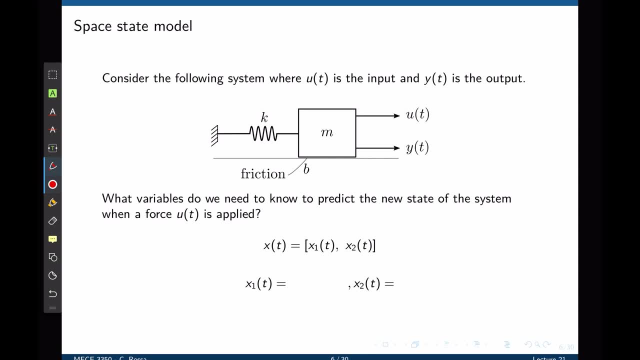 in order to predict the future behavior of the system given a current input. Let's start with an example. Consider the following mass spring damper system where u of t is the input- in this case a force- and y of t is the output, say position. What variables we need to know in order? 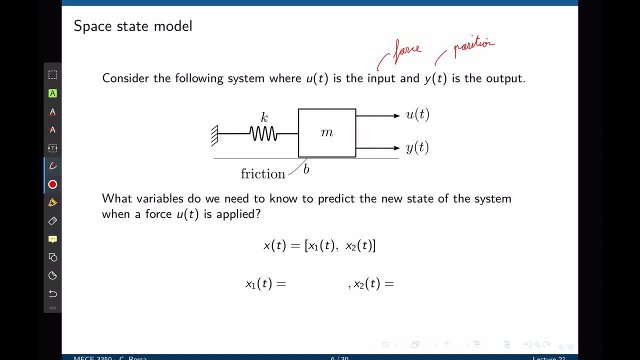 to predict the new state of the system when a force u of t is applied? The answer to this type of questions is typically found in the energy stored in the system. In order to predict the future behavior of the system, we need to know the current stored energy in that system. What? 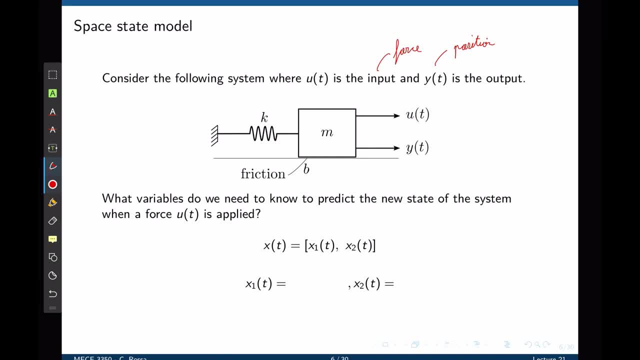 stores energy in a mass spring damper system. We have the potential energy stored in the spring- 1 half of kx squared- and we have the kinetic energy in the mass, which is 1 half of m times y dot. Thus the state variables can be defined as the displacement of the mass and the 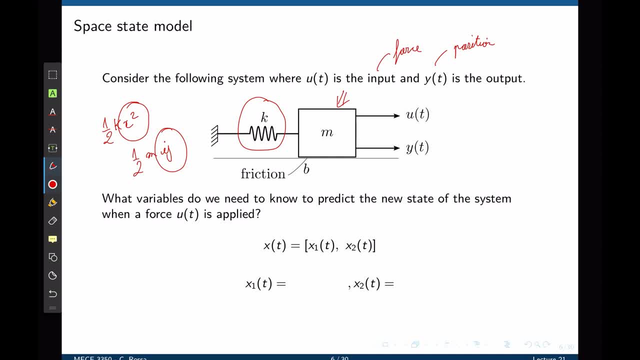 speed of the mass. These are the elements storing energy into the system. In order to predict the future behavior of the system, one needs to know the current position and the current speed. A good choice for the state variables, or therefore a good choice for the state variables, is the. 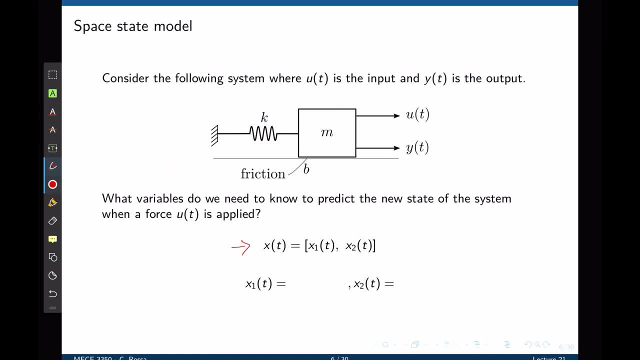 position and speed. We can now define the state space vector as x of t. The first entry is x1, the second entry is x2.. x1 we can define as the position and x2 is simply the derivative of the position or the speed. So x2 equals to y dot, which is the same as x1 dot, Once again, the state. 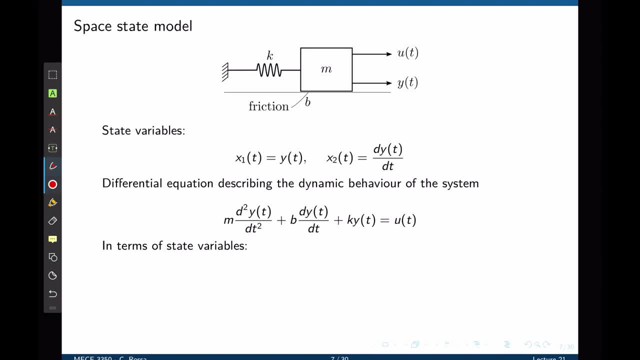 variables are: x1 equals to y of t position, x2 equals to the derivative of position. that is the same as x1 dot. Once we have defined the state variables, we can go back to the differential equation that describes the dynamic behavior of the system and rewrite that equation in terms of: 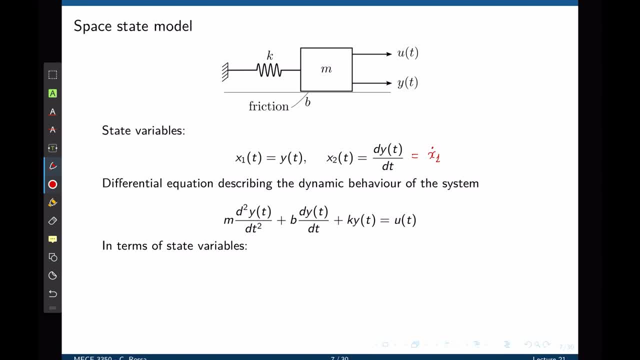 the state variables. We are going to use the lowest derivative possible for each variable in order to represent these equations. And remember that the objective here is to use first order differential equations. only Newton's law says that the sum of all forces acting on the mass is equal to m times. 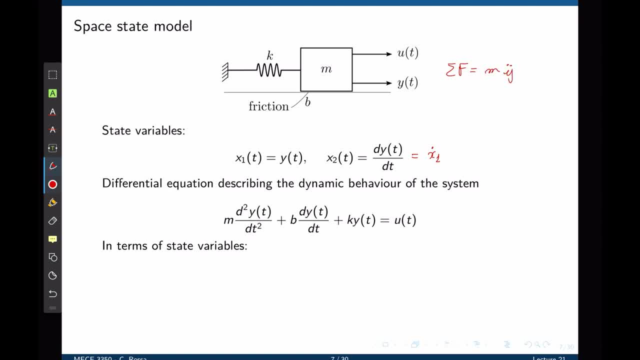 y double dot. The sum of all forces acting on the mass is equal to m times y double dot. The sum of all forces here is simply the spring force, k times y minus friction force, that is B times Y dot. And they act on in the opposite direction, as U. 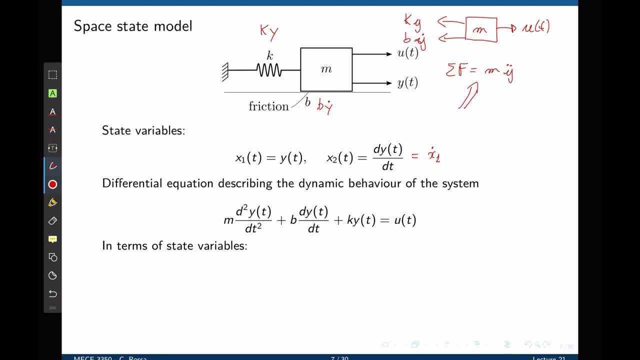 But now applying Newton's law to this system, here we get a well-known equation for the mass spring-grease damper system. We can now represent this equation using the state variables we have defined. Remember that our objective is to limit this to. 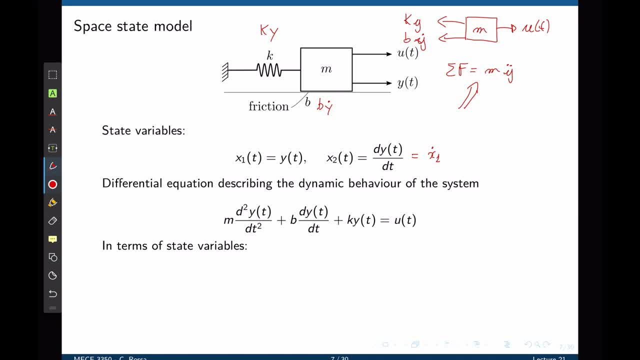 first-order equations. The first term is My estátua dot. In terms of the state variables, this can be described as m times x2 dot. So if x2 equals to y dot, x2 dot equals to y double dot, Why not write m x1 double dot? This is also a valid 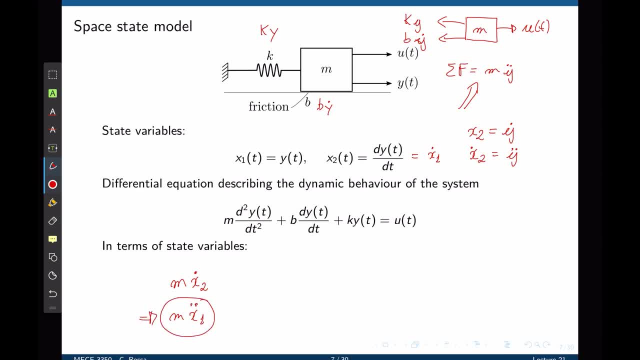 representation. but now we are dealing again with second order differential equation, And our objective is to limit all this to first order differential equations. Hence x2 dot is a better choice. Now let's move on to the second term, b times, dy dt or y dot. We have two choices here. 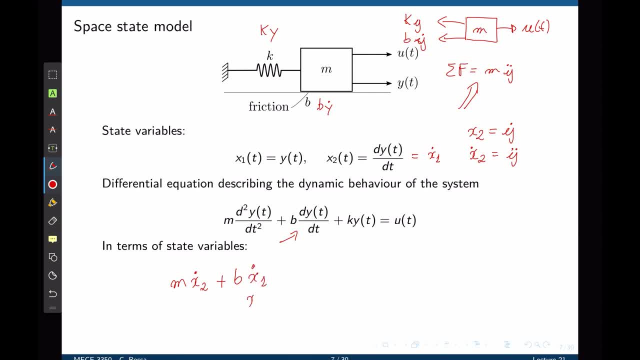 We can write x1 dot or we can write x2.. When you have multiple choices, it is always convenient to go with the lowest derivative, In this case x2.. We have b times x2, which is, again remember, is y dot Plus k times y of t, and y of t was defined as x1. And this is equal to u of t. 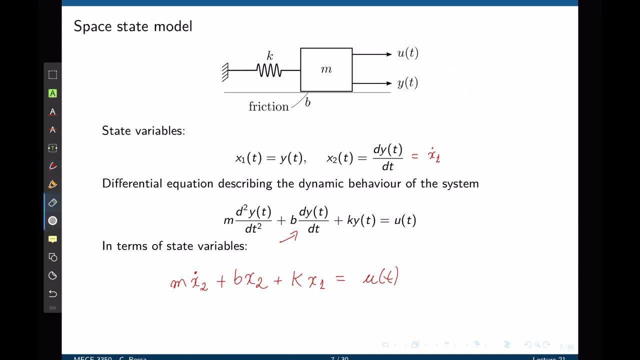 the input force. Now that we have the dynamic equation in terms of the state variables, we need an equation for all states and for all the derivative of those states. For example, x1 is known to be y of t And we know that x1 dot is x2.. We also know that x2 equals to x1 dot. 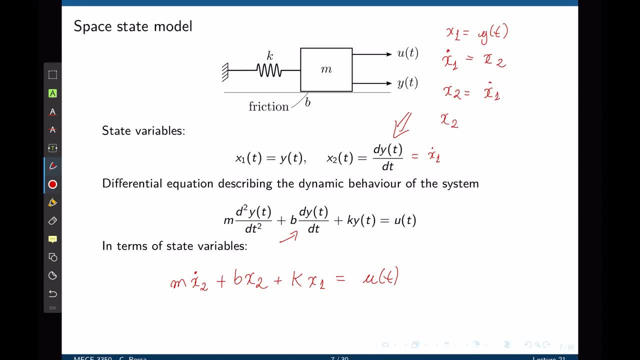 is the same equation. But now what is x2 dot? We can find x2 dot by isolating x2 in this equation here. So x1 dot becomes u of t divided by m minus b over m x2 minus k over m x1.. And you see. 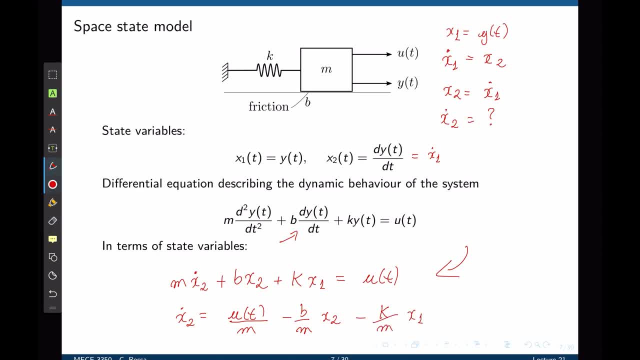 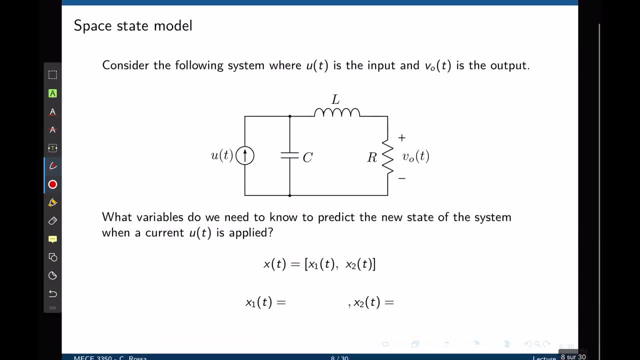 that again, this is a first order differential equation, And once you have all these equations, we can combine them in a matrix. We'll see that later, But before we do that, let's look at another example. Now let's shift the focus to an electrical system. Consider the following system. 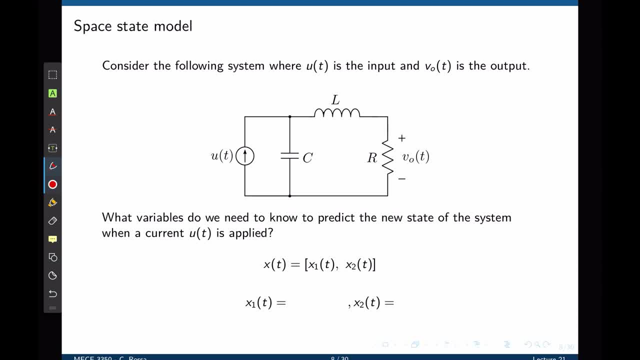 where u of t is the input current and v0 is the output. What states do we need to know to predict the new states of the system? We can use the following system to calculate the new states of the system. We can use the following system to calculate the new states of the system. We can: 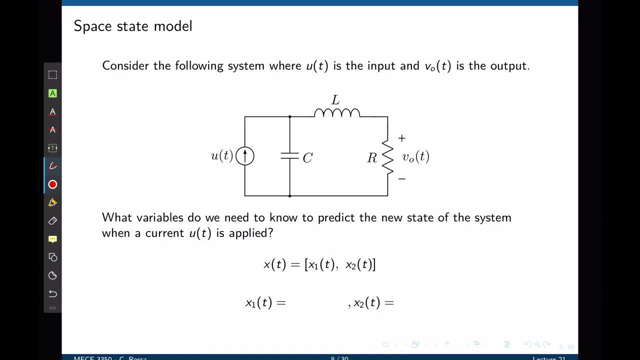 use the following system to calculate the new states of the system. We can use the following system when a current u of t is applied. Again, the answer to that question is typically found in the energy stored in the system. Which elements in this circuit can store energy? The inductor and. 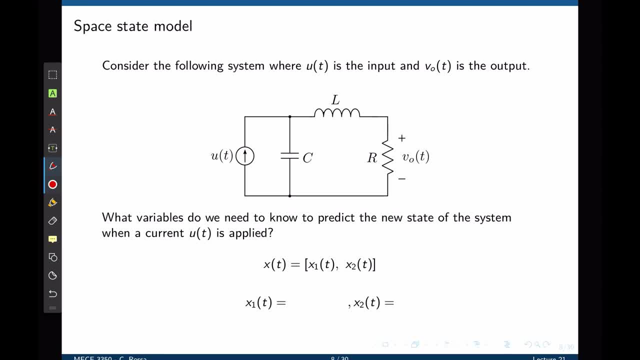 the capacitor. The inductor stores energy in the form of a magnetic field, And the energy stored in the inductor is a function of the current. through the inductor, The capacitor stores energy in the form of an electrical field, And the energy is a function of the voltage. 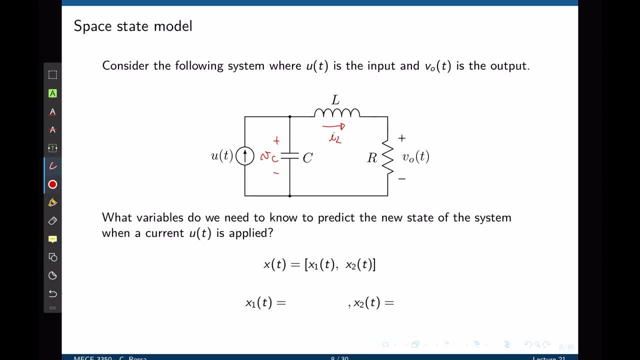 across the capacitor, Hence a good choice for the state. variables are the voltage of the capacitor across the capacitor and the current across the inductor. If you write the equations describing the behavior of this system, this is a second-order differential equation, Hence we'll need two state. 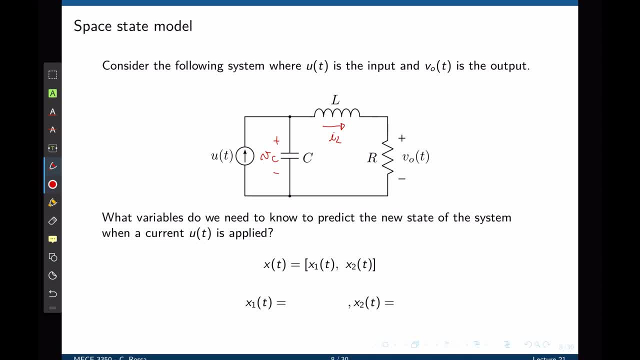 variables, And those are the current and the voltage as defined. If the system turned out to be a third-order differential equation, then you would need three state variables. We cannot define the state vector here. x of t, x1 and x2, where x1 is the voltage across the capacitor, vc and 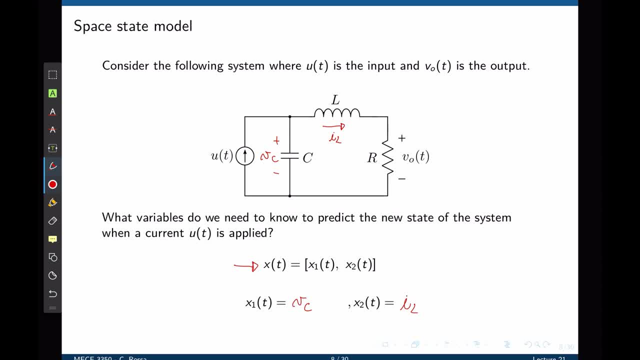 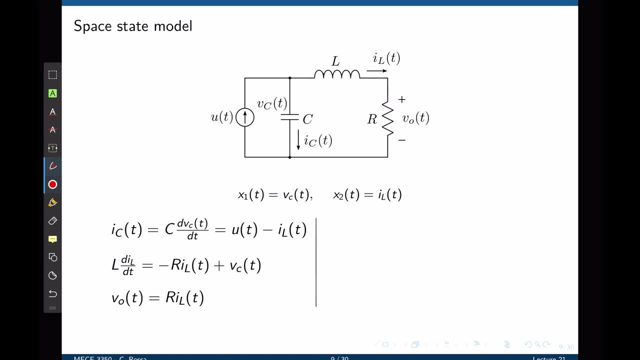 x2 is the voltage across the capacitor vc. So we can use the following system to calculate the new current with respect to current across the inductor il. The output of the system is v0.. We can now apply Kirchhoff's law to the system. to model it, We can start by specifying: 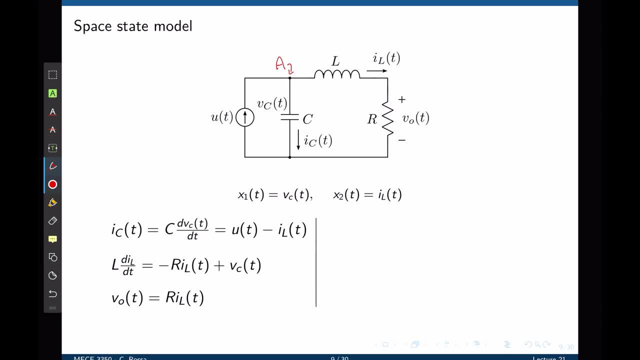 the current at node A. The current that we have here is the input current, u of t, which is equal to ic, the current through the capacitor plus il. This means that the current through the capacitor is u of t minus il. The current through the capacitor is also known as: 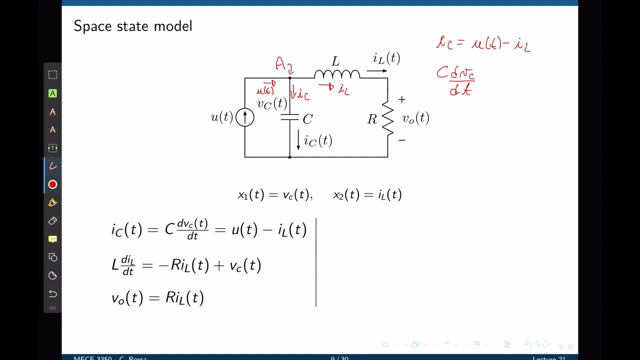 the derivative of the capacitor. The derivative of the capacitor is u of t minus il. This means that of the voltage across the capacitor, And this is U of T minus IL. And here we see one state variable, the second state variable and this is the input to the system. This is what gives the 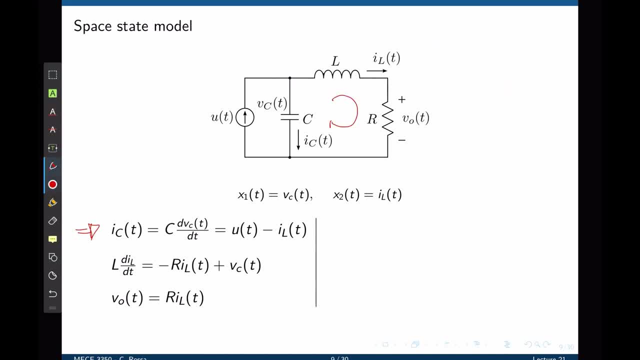 first equation. Next we can do Kirchhoff's law. in this loop, The voltage across the inductor is L times the IL DT, the derivative of its current. The voltage across the resistor is R times IL And the voltage drop across the capacitor is negative, VC. Negative because the sign of this 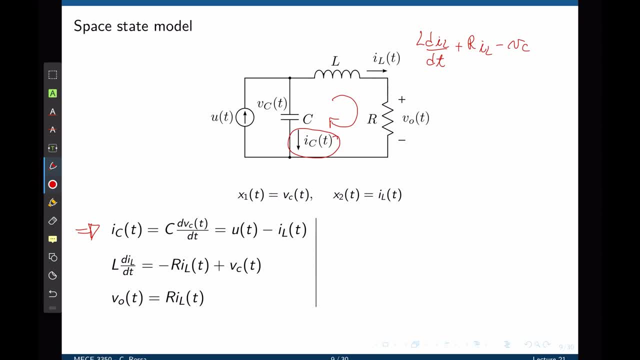 current is defined as going downwards And this is equal to zero. Remember that our state variables are IL and VC. We now need to define the equations for DIL, DT and DVC over. DT. For this one we already covered, This is the expression for the derivative For DI- DT. we can now use this: 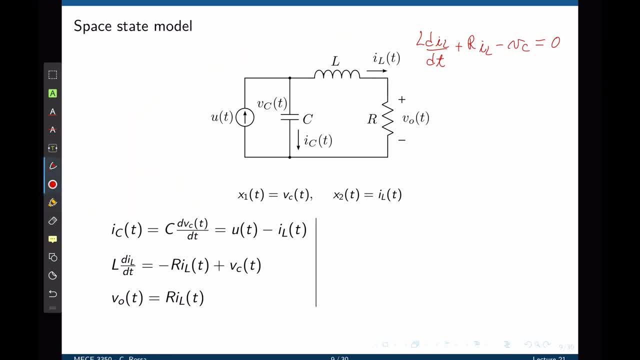 expression. By rearranging this equation, we get this: DIL DT equals to VC minus IIL. Finally, the output voltage V0 is simply IL, the state- one of the state variables- times R. And this is the last expression here. Now that we have all these expressions, we can write them as a function. 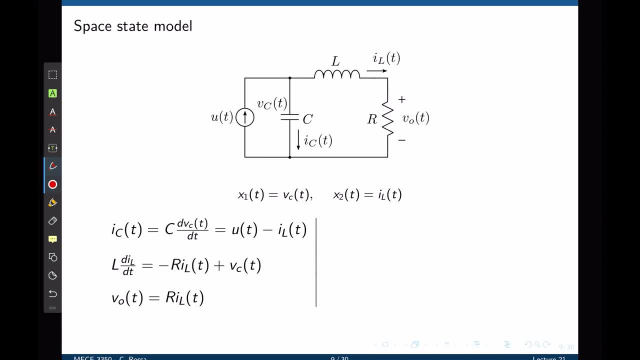 of the state variables. Let's start with the first equation. DV DT is simply X1 dot. We can now write that X1 dot is U of T minus IL, And this is the last expression here. Now that we have all these expressions, we can write them as a function of the state variables. Let's start with the first. 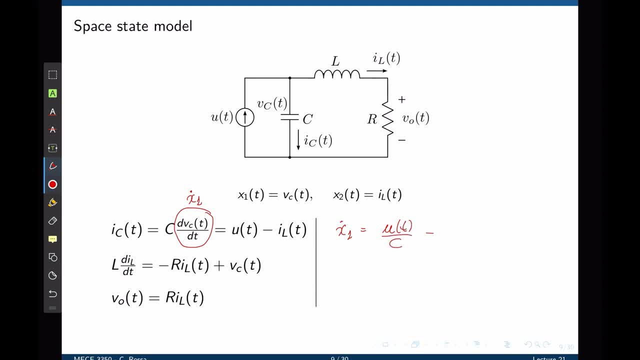 equation U of T over C minus IL over C, And IL is X2.. Now, moving on to the second expression, we have DIL DT. This is clearly X2 dot, And X2 dot then becomes negative R over L times IL. 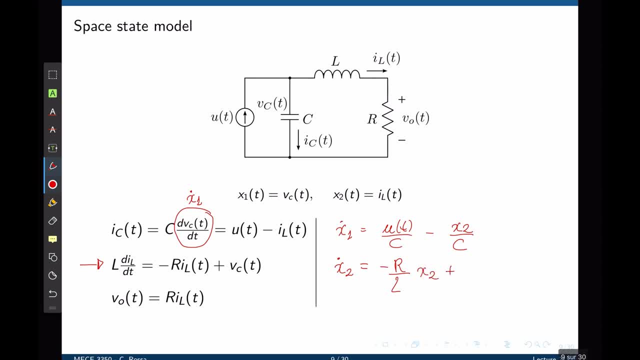 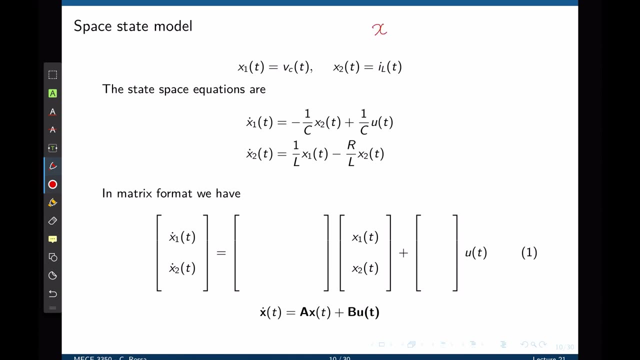 which is X2, plus VC, which is X1.. And the output is simply R times IL, which is X2.. Now that we have these expressions, we can put them in a standard form for a state-space model, And here is the state-space equation. We now wish to express these functions as a first-order. 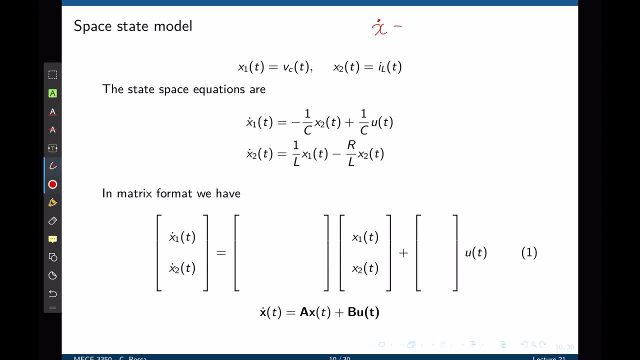 differential equation: X equals to X. dot equals to A times X plus B times U. X dot is the derivative of X and X is the state vector. A and B are matrices to be determined based on these coefficients, And U is the input to the system. Now let's see how we can write these expressions in this format. 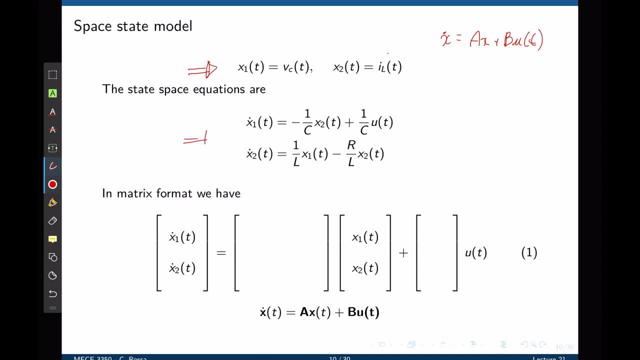 Here we have the definition of the state variables and here we have the derivative of the state variables. Two equations are the equations we got in the last step in the previous slide. Remember that X is X1, X2.. So X dot is an element-wise operation. We have X1 dot, X2 dot. 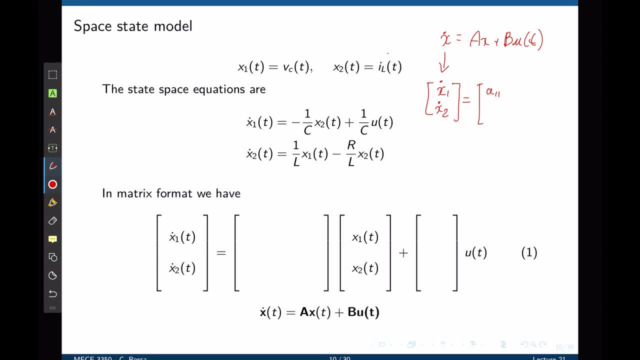 This is equal to A. In this case, A will have to be a 2 by 2 matrix. X is again X1, X2.. B is a 1 by 2 matrix and we have this times U of T. So now our job is to find these A's and B's. 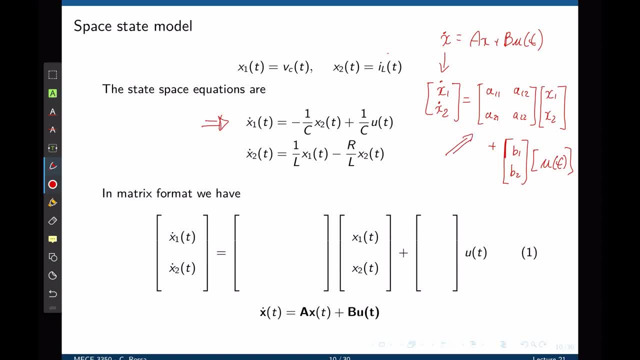 So now let's look at the first equation for X1 dot. Nothing in this expression multiplies X1 dot, So the first cell here is 0.. What multiplies X2 dot? X2 dot is multiplied by negative 1 over C. right here, If we move on to the second row. 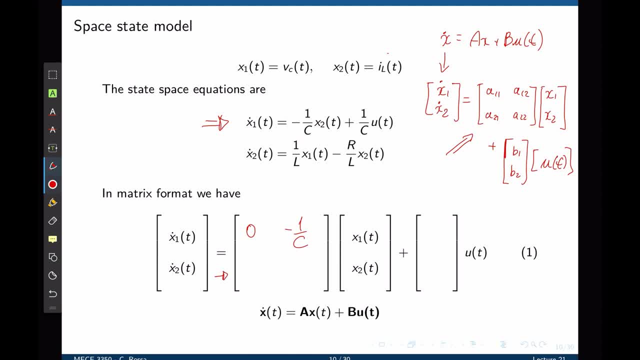 now we are looking at X2 dot. What multiplies X1?? Well, that is 1 over L. right here, That multiplies X1.. And what multiplies X2? That's negative R over L. Now we can go to our matrix. 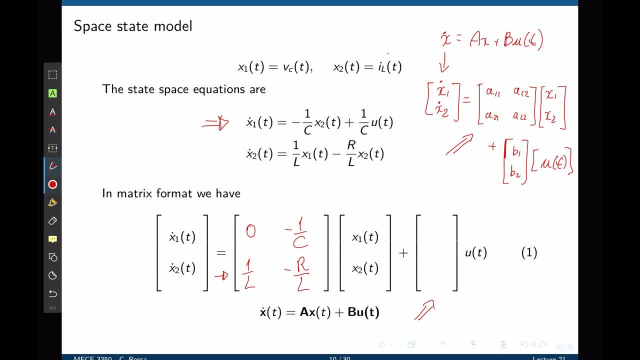 Now we can go to the second part of the matrix, In which of these expressions we see the input. Well, the input is only shown here, So clearly, for X2 dot. there is no direct relation between X2 dot and U of T, So that term is 0.. And the term right above it is 1 over C. 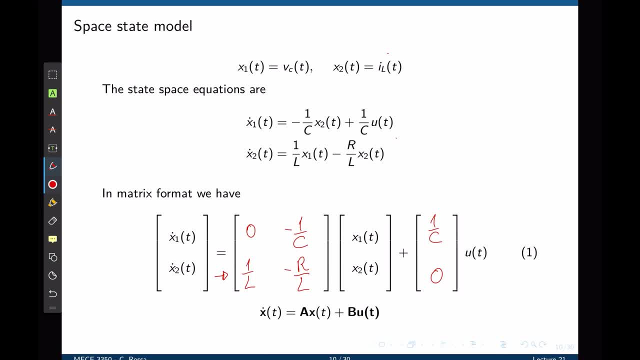 So now notice that if we expand this matrix, we'll go back to the exact formulation we had here, And this matrix representation is a representation of dynamic model of the system using only first-order differential equations. The first step in this process has this Center: hyperbolic. 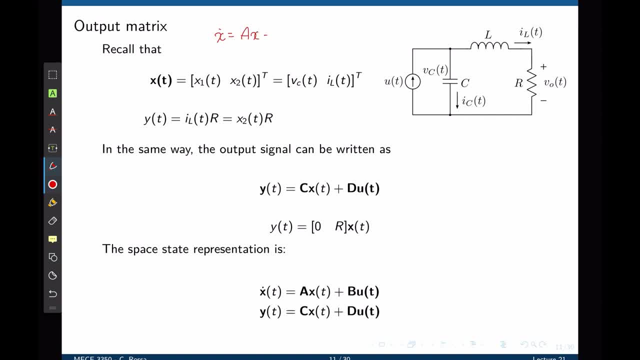 form we just saw. x dot equals to a times x plus b times u. So this is the relation between the states of the system, their derivative and the input. What about the output of the system? For the output of the system, we need a new set of equations and in this case we are going to write. 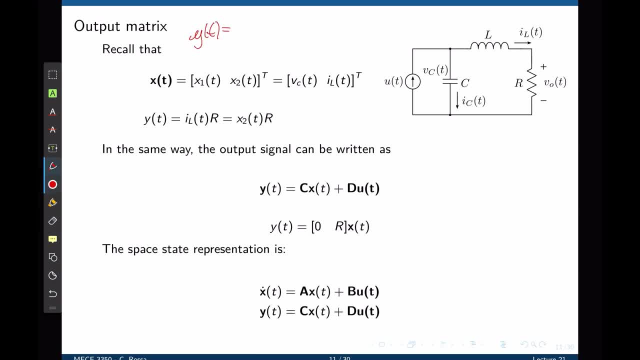 the output of the system, which is defined as y, as c times x plus d times u of t, x are the states of the system, u is again the input of the system and x is the state variable. once again, Remember that we define the output of our system to be the voltage across the resistor, that is, v0 or il times. 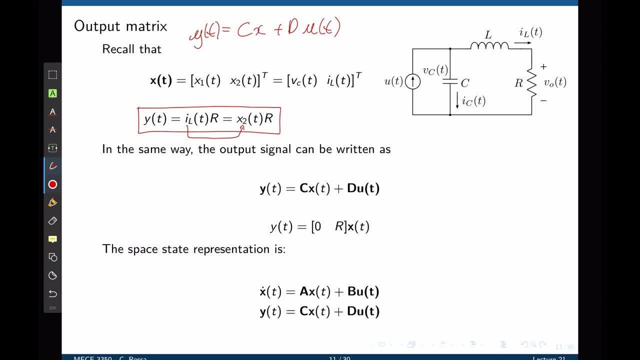 r and il being x2.. This is the representation of the output voltage. If you now use the standard formulation for the output, voltage, y of t is equal to a matrix that to be determined, that is, the matrix c. We see that the output is not directly related to x1, it's only a function of x2.. So the first 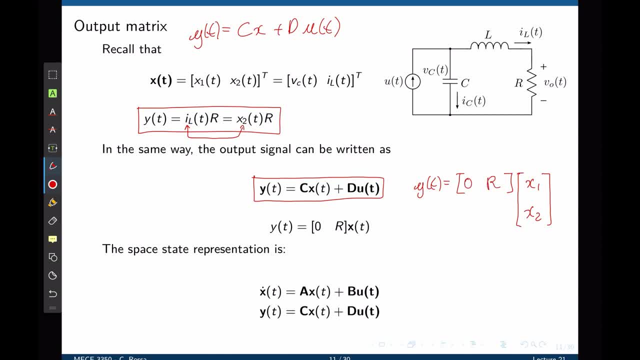 element here is 0 and the second element is simply r, And this multiplication recreates this expression here Plus d times u, and you see that u of t does not show up directly in the expression of the output. so d in this case is 0.. With these two sets of equations we can now represent the 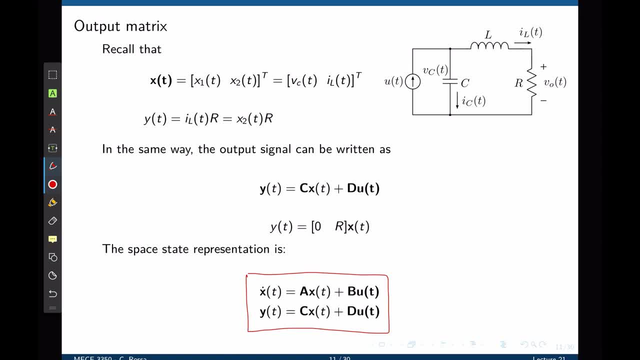 system entirely Using only first order differential equations. The first equation again relates the derivative of the states and the states with using these two matrix with the input to the system. The second set of equations gives the output of the system. given the current state of the system, the input provided.